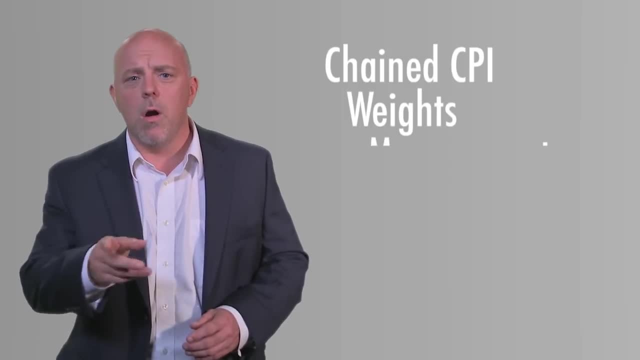 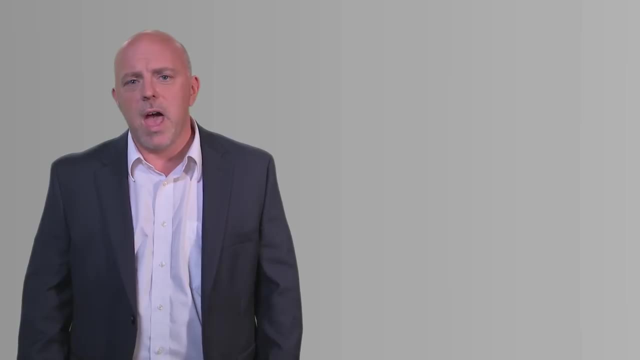 consumer goods and services in the Chained CPI are more current than the weights used for the U or the W, For example in the CPI-U and W for 2015,. the categories of goods and services that consumers buy are based on expenditure surveys conducted in 2011 and 2012.. So those weights are: a few years old. Consumer behavior can change a lot in just a few years. Consider telephones: In recent years the use of landlines has fallen dramatically as self-in use has correspondingly increased. The final Chained CPI will correspond more closely to how consumers are currently. spending their money. A second difference between the Chained CPI and other CPIs is that the Chained CPI reflects how consumers respond to changes in relative prices. For example, suppose the price of beef increases this month but the price of chicken falls, While some households may not change their 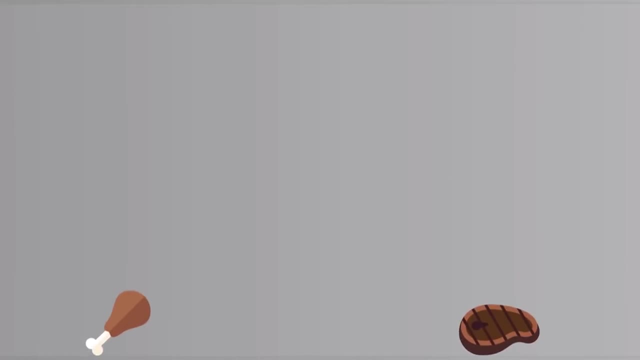 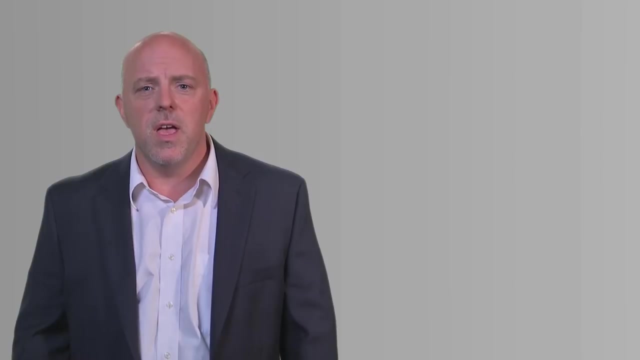 buying habits. as a result of this relative change, the U and W are the same. So the U and W are the same, but the price of chicken is different. The Chained CPI is unique among the CPIs we produce in that it explicitly takes into account how much consumers spend on goods and services in 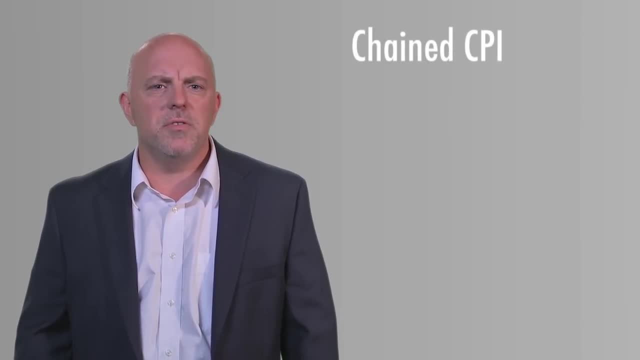 both months. In short, since the Chained CPI uses more current consumer spending patterns and is designed to reflect changes in actual consumer behavior, the Chained CPI is designed to be a closer approximation to a cost-of-living index than the CPI-U or the CPI-W. Over time, the Chained CPI tends to increase at a slightly lower rate than other measures of consumer inflation. For example, over the 12-year period from December 01 to December 13,, the Chained CPI rose at an average annual rate of 2.11%, compared to 2.33% for the CPI-U. While we can 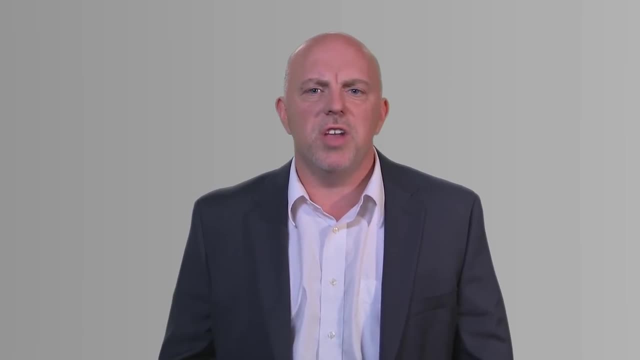 say that the Chained CPI is a better general or overall measure of changes in the cost of living. there is a limitation of the Chained CPI that people should be aware of when considering which measure of consumer inflation to use. Namely, the Chained CPI is. 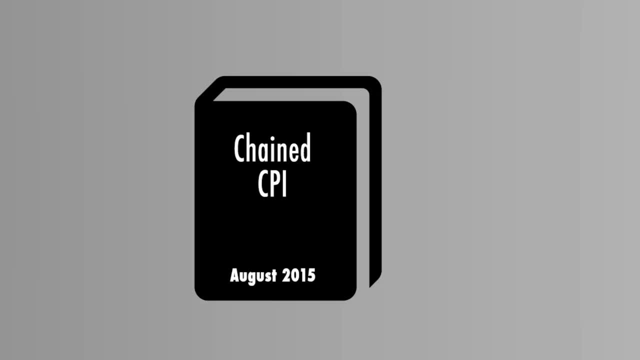 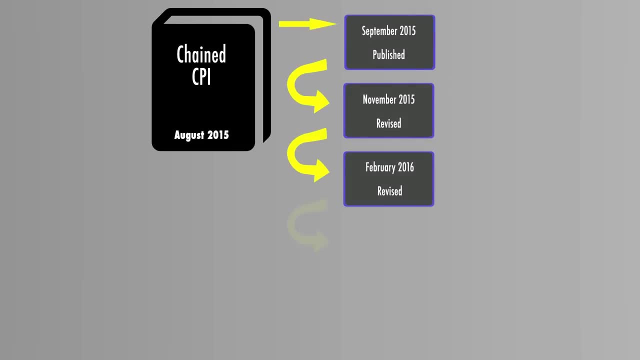 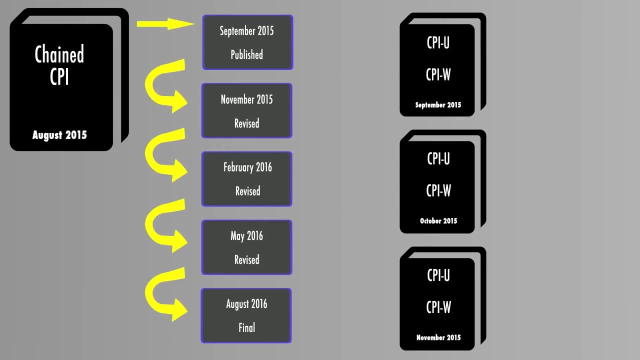 subject to four quarterly revisions. For example, Chained CPI indexes for August 2015 are initially published in September 2015, revised each of the next four quarters and aren't published as final until August 2016.. In contrast, when we publish the CPI-U and W indexes each month, they are considered final when first issued. The final Chained CPI needs both current prices and current spending patterns. While we can go to stores and collect the prices right away, it takes many months to determine how much consumers are spending on various items each month. Finally, a potential limitation of all three inflation measures: the CPI-U, CPI-W. 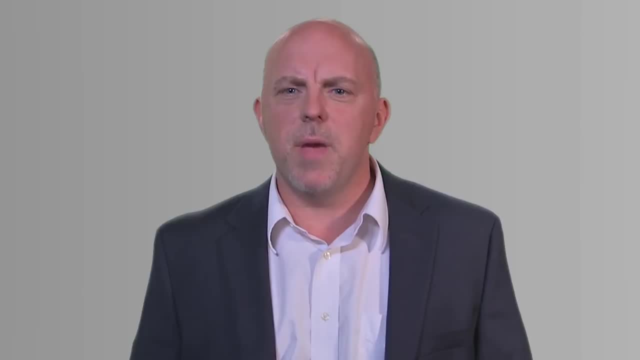 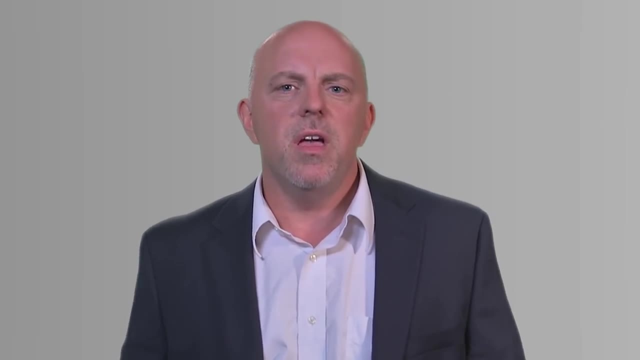 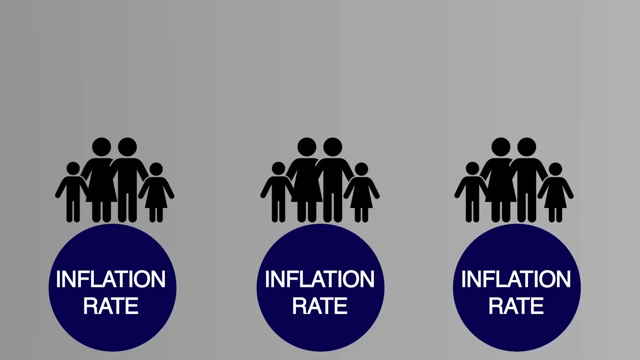 and the Chained CPI is that they might not be the best measure of the changes in cost of living for each and every American. All three measures are merely averages. They measure changes in the cost of living for consumers or for urban wage earners and clerical workers, Each individual family. 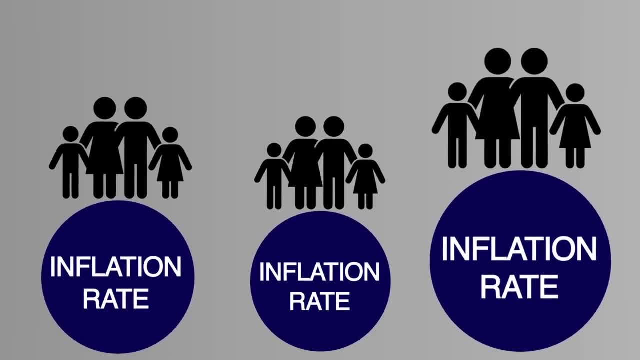 on the other hand, has its own personal inflation rate. Indeed, these three CPIs may not be representative of specific individuals or individual families, or even for specific groups of people such as senior citizens. In summary, a goal of the Bureau of Labor.